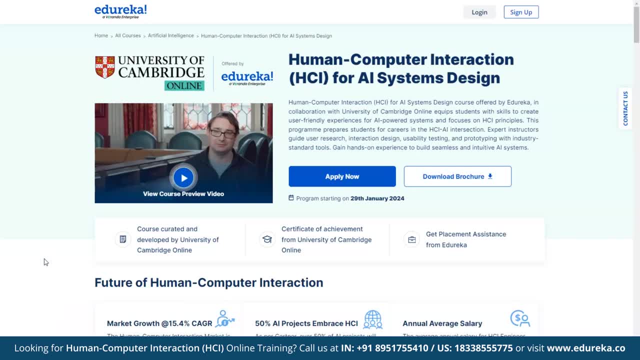 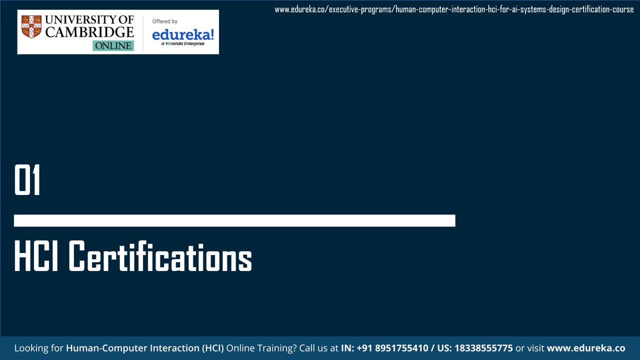 the Edureka website for training and certification courses, the link to which is in the description box below FCI Certifications. Companies are in search of candidates with skills such as user-centered design, user research and technical skills. These skills contribute to the ability of FCI professionals to create interfaces and 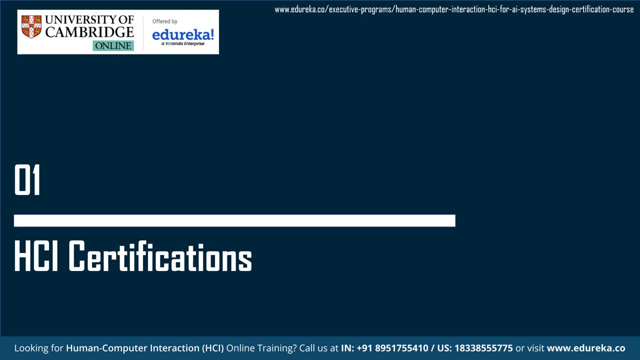 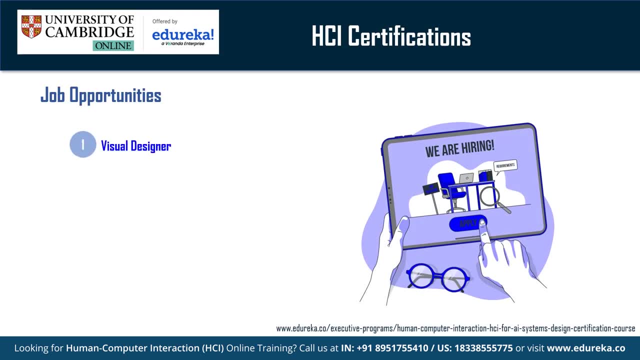 systems that enhance user experience. Some in-demand job roles in the field of FCI include visual designer, user experience researcher, accessibility engineer, cognitive systems engineer and software engineer. According to Sixfigurecom, the average salary for a human-computer interaction professional is $1.5 billion. FCI Certifications Companies are in search of candidates with skills such as user-centered design, user-centered design and technical skills. These skills contribute to the ability of FCI Certifications Companies to create interfaces and systems that enhance user experience. The average salary for a human-computer interaction professional is approximately 21.7 lakhs per. 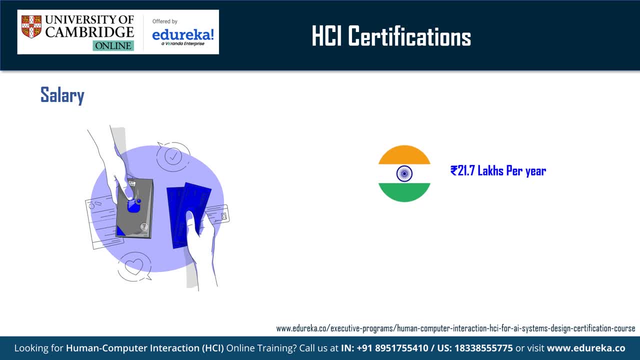 annum. in India, The estimated average paid for a human-computer interaction professional is approximately $249,000 per annum. in the United States, FCI professionals are in high demand today and are likely to persist as organizations strive to strengthen their user interface interactions. Certifications are an important 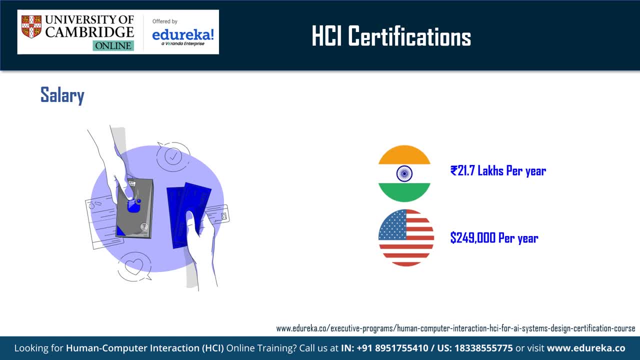 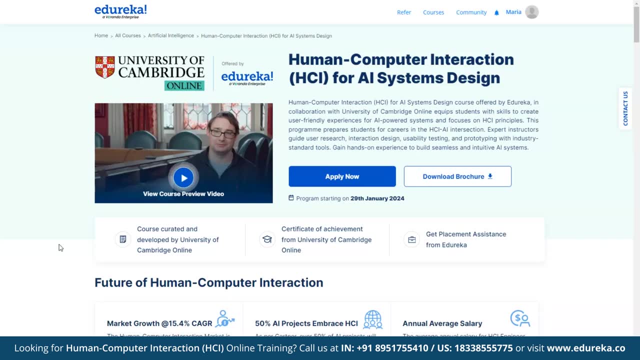 aspect of landing a job in human-computer interaction. The Human-Computer Interaction for AI Systems Design course, offered by Edureka in collaboration with the University of Cambridge Online, is the first step to begin your HECCI journey. This course equips students with skills to create user-friendly experiences for AI-powered 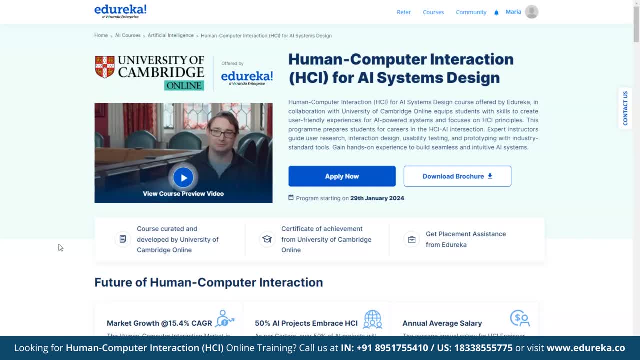 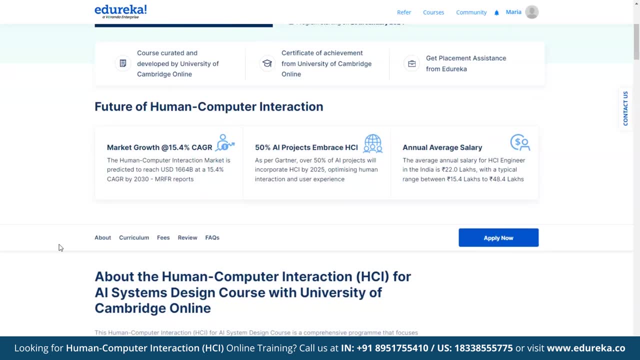 systems and focuses on HECCI principles. This program prepares students for careers in the HECCI-AI intersection. Once you finish the Human-Computer Interaction for AI Systems Design course, you will be able to start your career as a human-computer interaction professional. 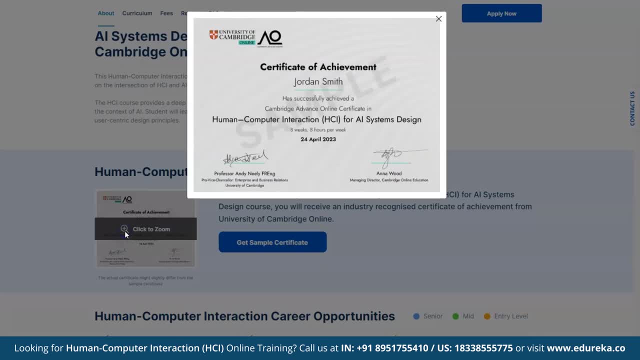 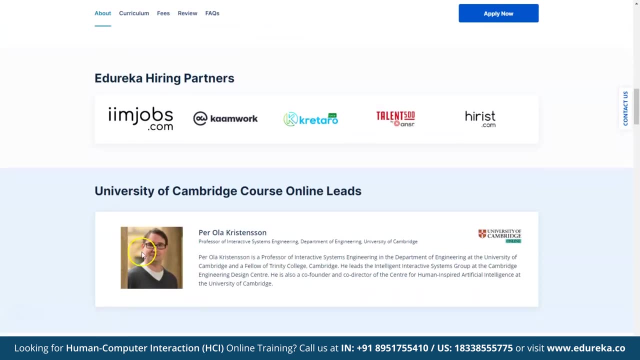 You will get a certificate from the University of Cambridge Online, which is well respected in the industry. Taking the lead at the University of Cambridge course online is Professor Per Ola Christensen. He serves as a Professor of Interactive Systems Engineering within the Department of Engineering at the University of Cambridge and is additionally 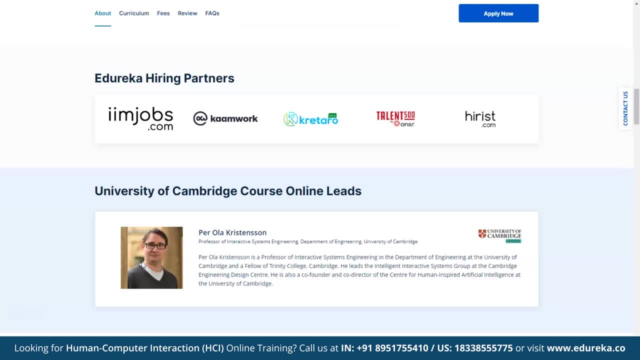 recognized as a Fellow of Trinity College, Cambridge. To know more details about the course curriculum and skills it covers, please visit the website at wwwinteractive-systemscom. Thank you. So why is human-computer interaction important? User-Centered Approach. 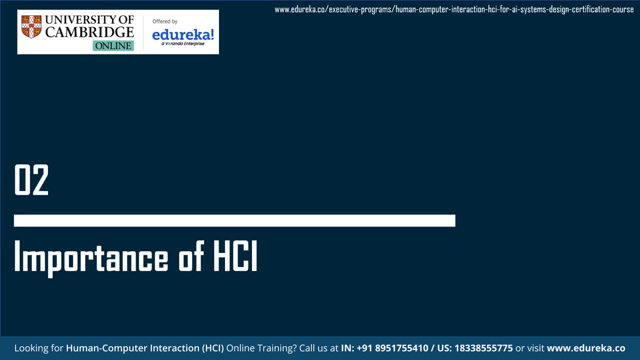 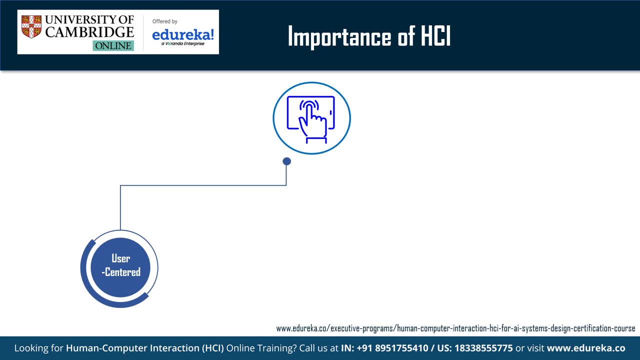 HECCI focuses on a user-centered design approach. This approach results in products and systems that are more user-friendly and align with the expectations of diverse user groups. Breaking Down Complex Technology, HECCI is essential for designing interfaces that allow users to navigate and interact with complex systems efficiently. So these interfaces can help users manage advanced 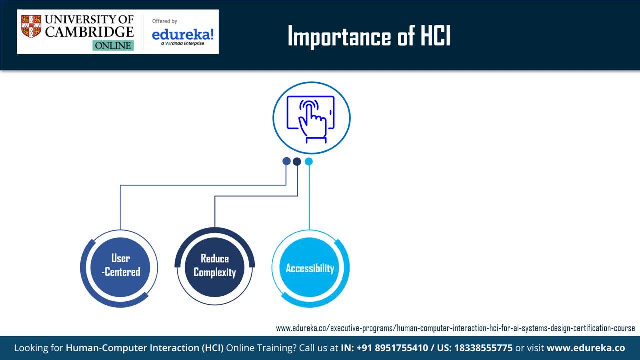 technologies with ease. Accessibility for Diverse Users: Designing interfaces that are accessible to individuals with varying levels of technological expertise, as well as accommodating different physical and cognitive abilities, is a key aspect of HECCI. Rise of Wearable Technologies, With humans being highly dependent on smartphones, tablets and smartphones, HECCI is a key aspect. 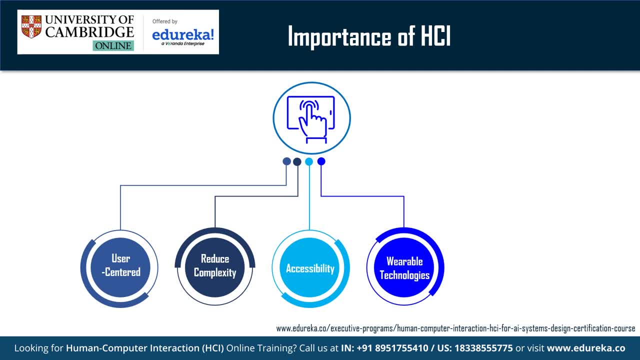 of HECCI. HECCI is crucial in designing interfaces for different interaction methods. Ensuring a seamless user experience on these devices is a finish Continuous Technological Innovation. HECCI remains relevant as technology continues to advance. Designing interfaces for emerging technologies such as artificial intelligence and the Internet of Things requires expertise. 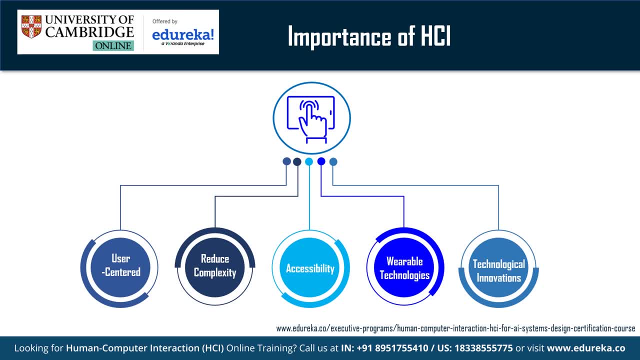 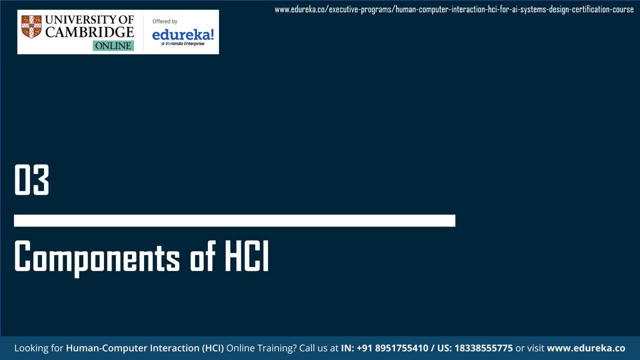 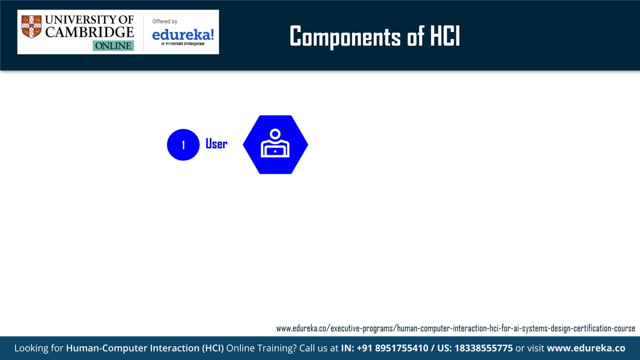 in understanding how users interact with these technologies and how to make these interactions meaningful. Components of HECCI. The main aim of HECCI is to make software websites, mobile applications and other systems more usable, efficient and enjoyable for users. Human-computer interaction involves various 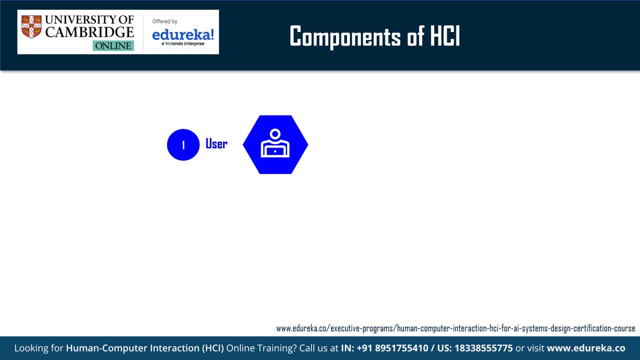 components that contribute to the design of interactive systems to make them more user-friendly and effective. The main components of HECCI include Users. Users are the individuals who interact with the computer system. Users have varying levels of preferences, behaviors and expectations. Tasks: Tasks represent the activities that users want to accomplish using the computer system. 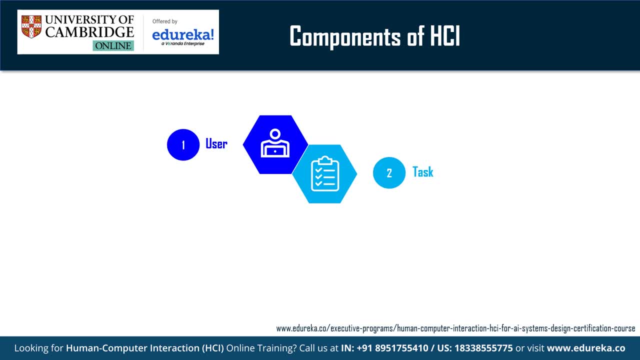 Understanding users' tasks is critical for designing efficient interfaces Systems. This component is the hardware and software elements that constitute the computer system. This includes devices such as computers, smartphones, tablets and other applications. Interface: The interface is the point of interaction between the user and the computer system. 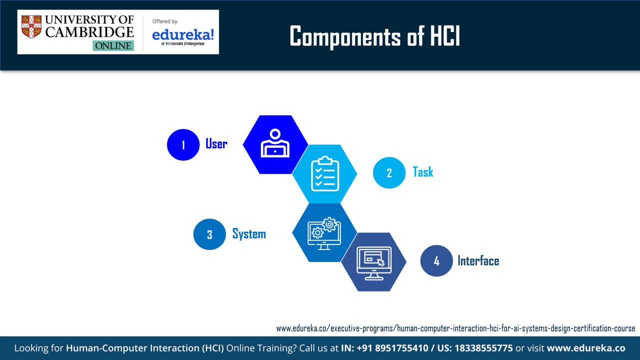 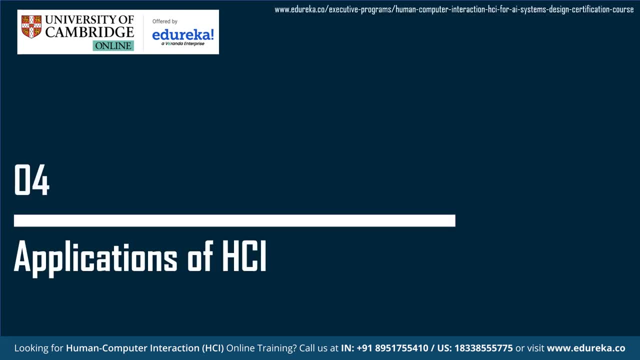 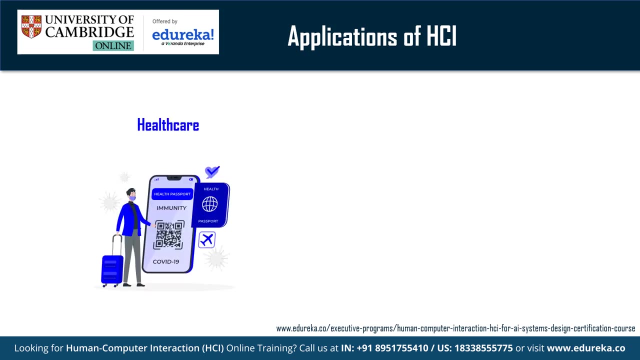 It includes elements such as screens, buttons, menus, icons and other design elements that the user and the system use for their interaction. Next, let's move on to the applications of HECCI: Healthcare. Human-computer interaction plays a crucial role in healthcare by improving the design. 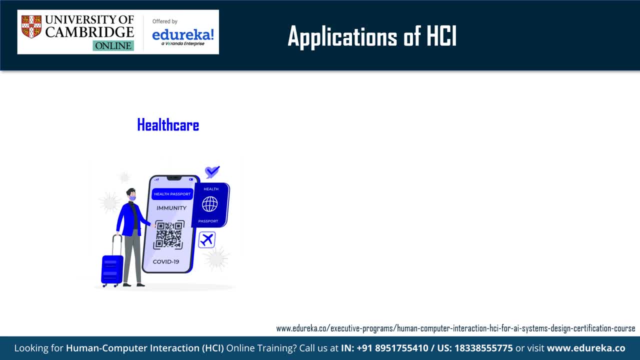 and usability of digital systems, interfaces and technologies used by healthcare professionals, patients and other stakeholders. HECCI principles are used in the design of EHR, that is, electronic health record systems, to ensure that healthcare professionals can easily navigate, input and retrieve patient. 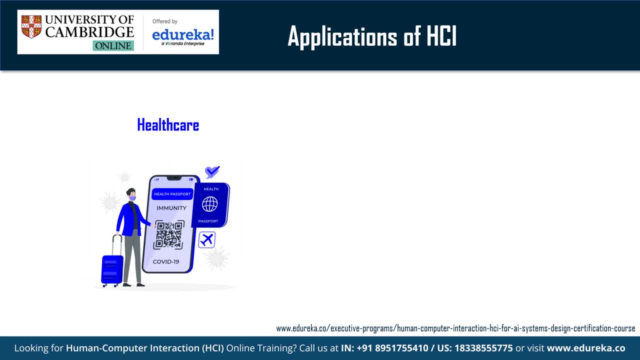 information. HECCI is applied in the design of interfaces for medical devices such as infusion pumps, monitoring equipment and diagnostic tools. These interfaces help healthcare providers use these devices more efficiently and minimize the risk of errors. HECCI is employed to design natural language interfaces that allow users to communicate. 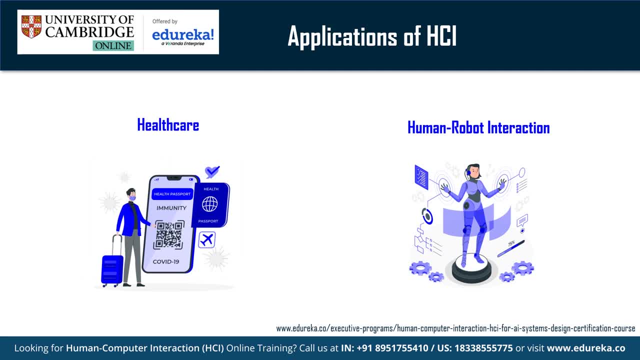 with robots through spoken or written language. This involves understanding user intent, processing natural language and communication. HECCI is applied in designing touchscreens and physical interfaces that allow users to interact with robots by tapping, swiping or using any other physical controls. 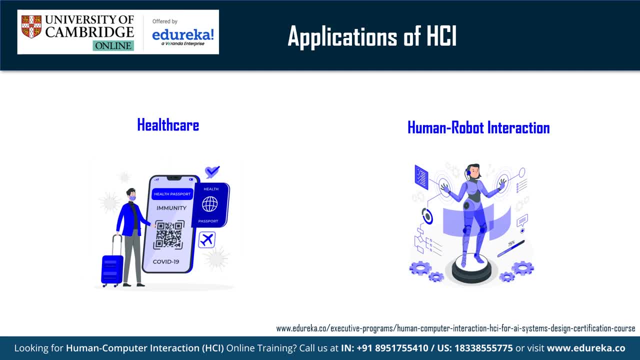 HECCI makes sure that interfaces need to be user-friendly and responsive. Human-computer interaction is essential for several reasons, as it plays a crucial role in shaping the design and usability of technology interfaces. HECCI is applied in designing touchscreens and physical interfaces that allow users to 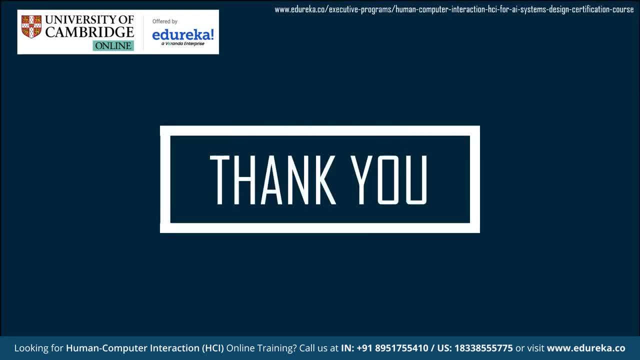 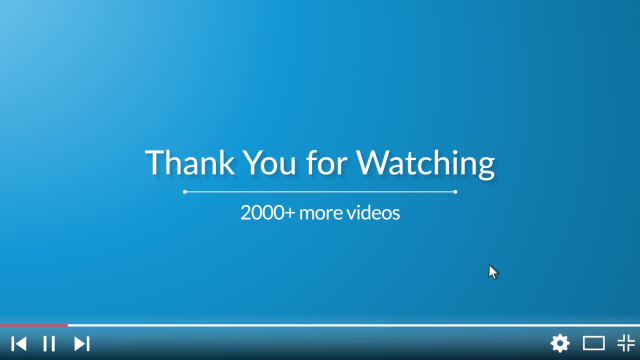 interact with robots by tapping, swiping or using any other physical controls. Human-computer interaction is essential for several reasons, as it plays a crucial role in shaping the design and usability of technology interfaces. So make sure to like and subscribe to our YouTube channel. 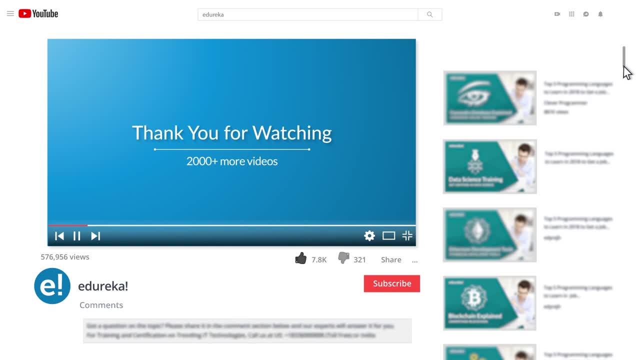 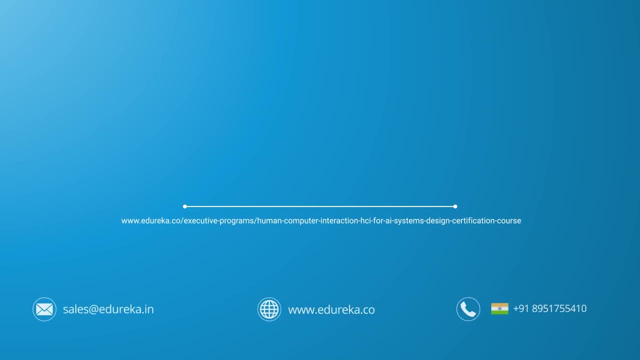 Thank you for watching and keep learning you.